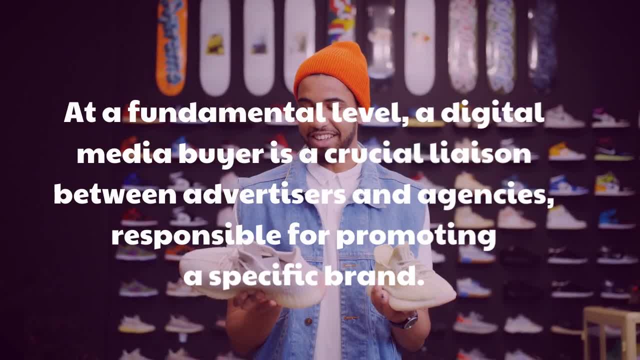 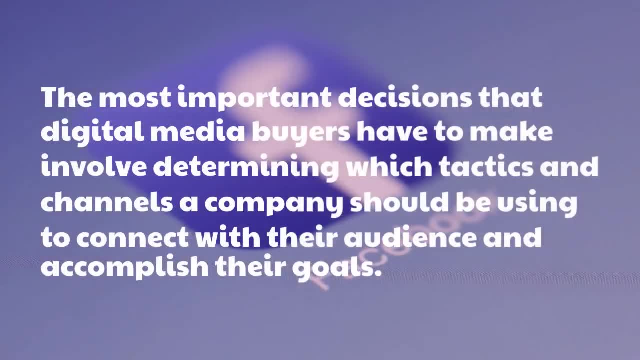 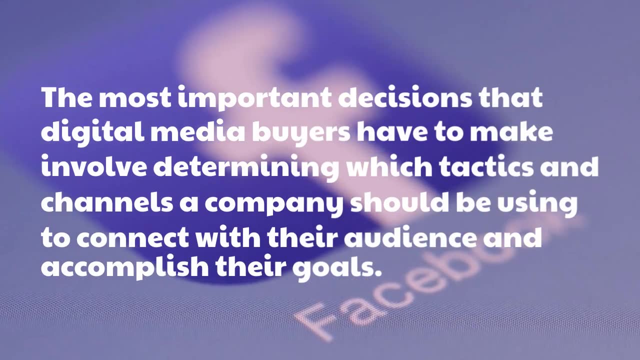 A digital media buyer is a crucial liaison between advertisers and agencies responsible for promoting a specific brand. The most important decisions that digital media buyers have to make involve determining which tactics and channels a company should be using to connect with their audience and accomplish their goals. 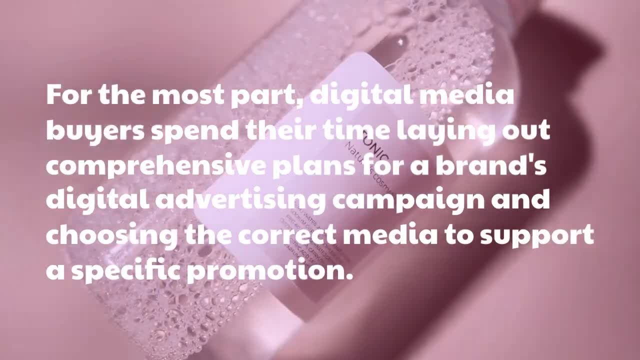 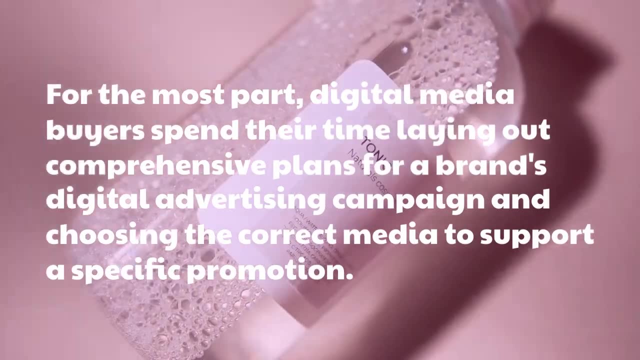 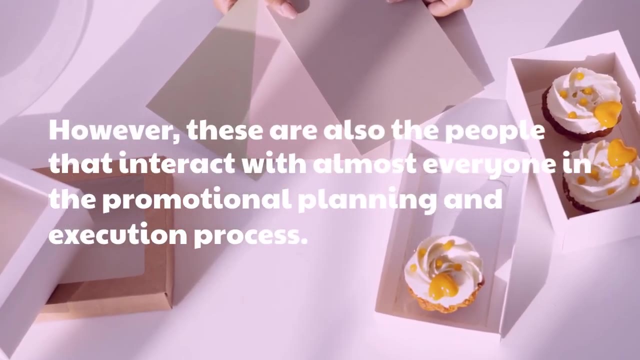 For the most part, digital media buyers spend their time laying out comprehensive plans for a brand's digital advertising business. They spend time analyzing campaigns and choosing the correct media to support a specific promotion. However, these are also the people that interact with almost everyone in the promotional planning and execution process. 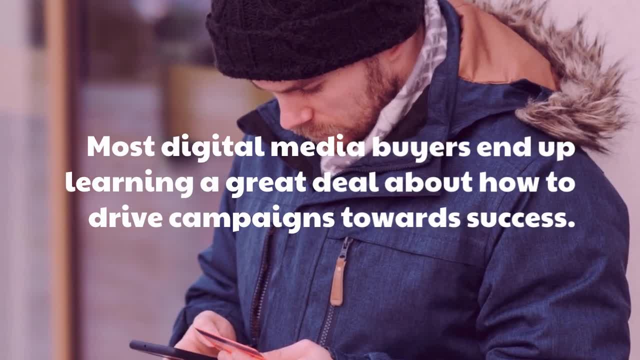 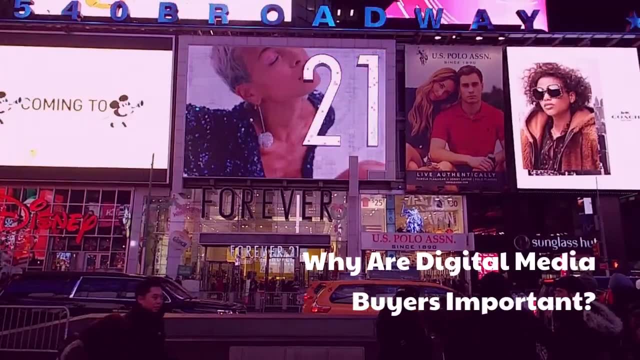 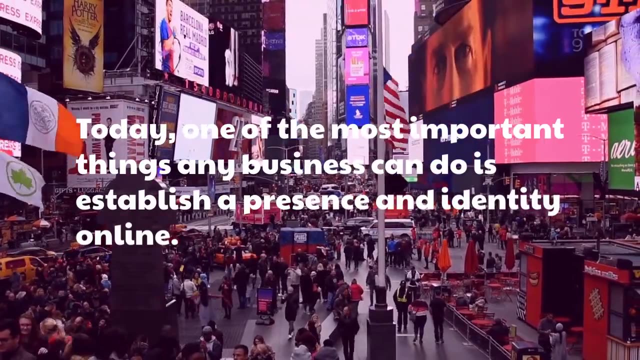 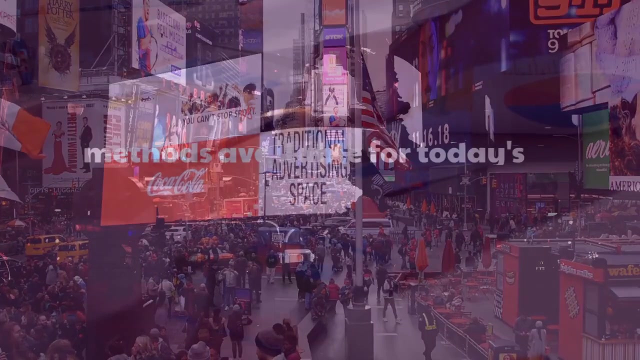 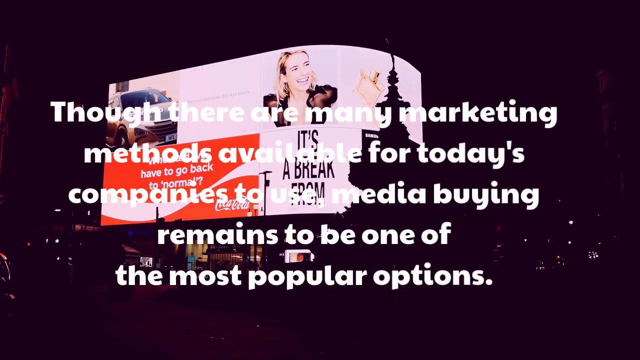 Most digital media buyers end up learning a great deal about how to drive campaigns toward success. Why are digital media buyers important? Today, one of the most important things any business can do is establish a presence and identity online. Though there are many marketing methods available for today's companies to use, media buying remains to be one of the most popular options. 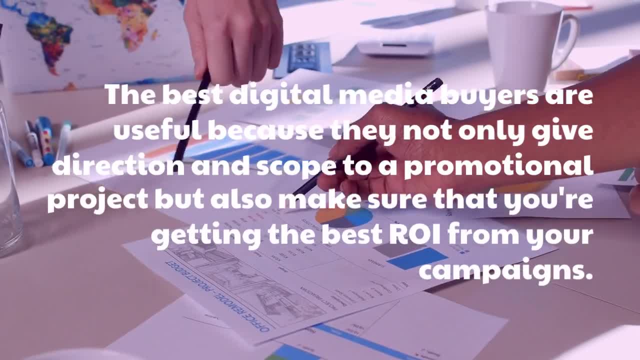 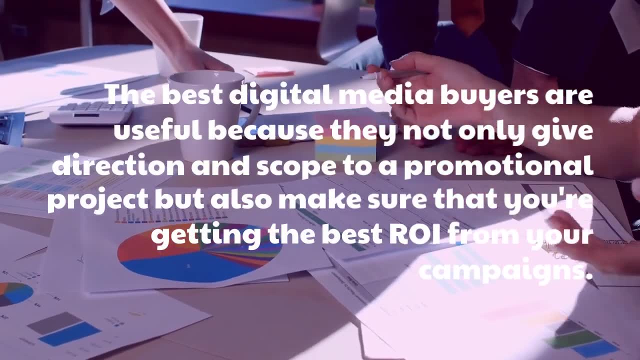 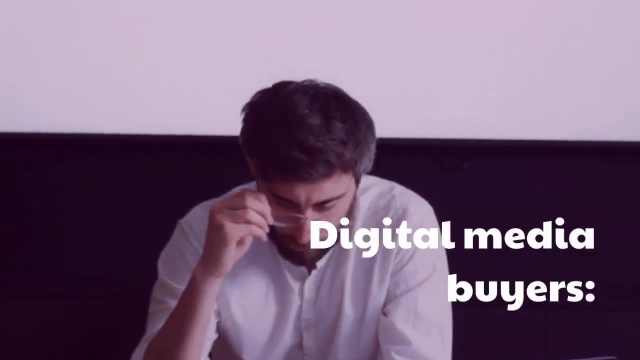 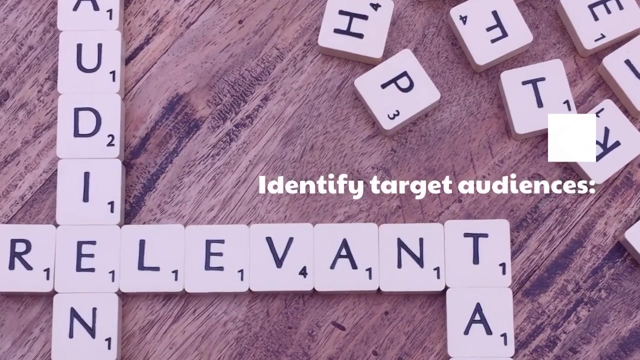 The best digital media buyers are useful because they not only give direction and scope to a promotional project, but also make sure that you're getting the best ROI from your campaigns. Digital Media Buyers Identify Target Audiences Before they ever get started with a bid. your digital media buyer will get to know you. 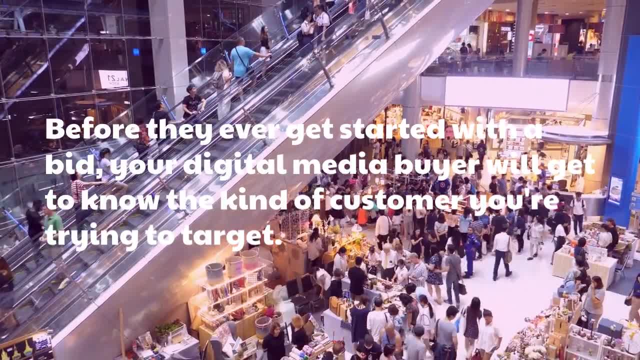 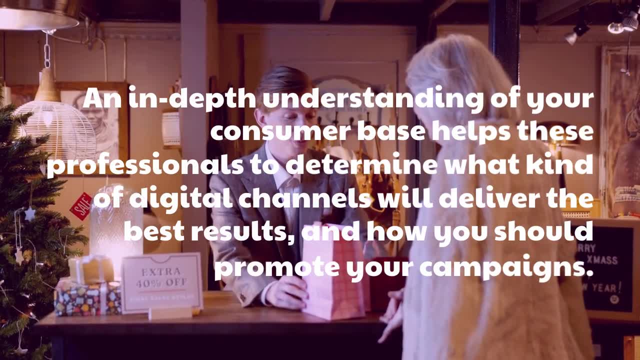 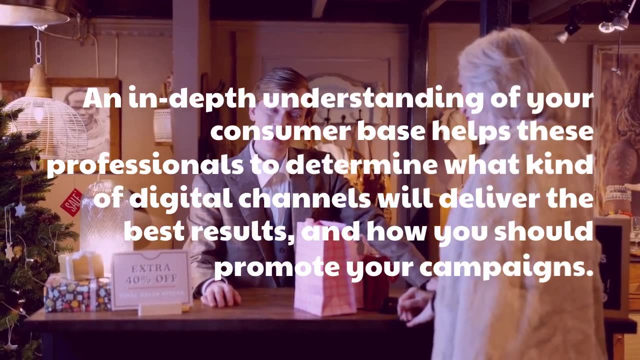 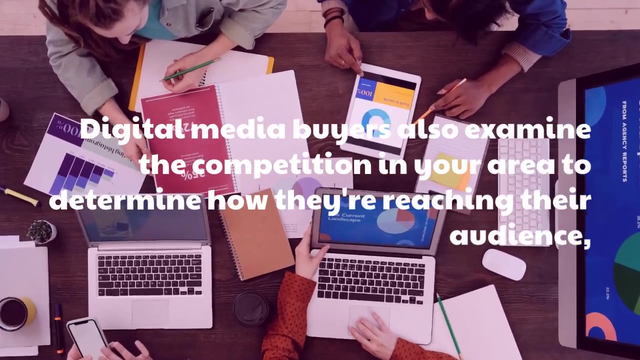 They will know the kind of customer you're trying to target. An in-depth understanding of your consumer base helps these professionals to determine what kind of digital channels will deliver the best results and how you should promote your campaigns. Audit the Competition. Digital media buyers also examine the competition in your area to determine how they're reaching their audience.